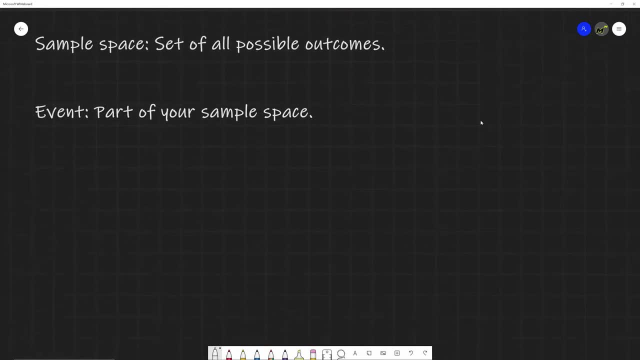 Now let's start out by identifying some of our sample space. Scroll down. Let's say we have a probability experiment that consists of tossing a coin and then rolling a six-sided die, Determine the number of outcomes and identify the sample space. Okay, what do we have going on? 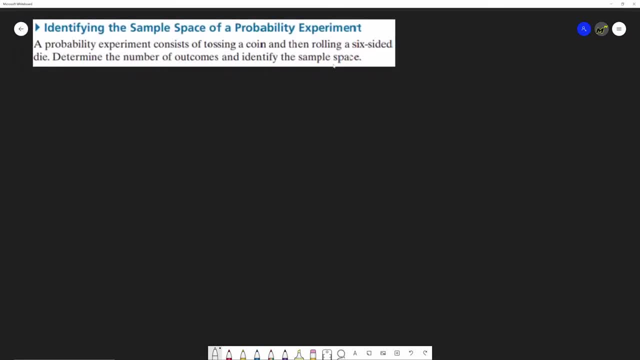 Okay, so we have- let's see- a six-sided die, and we need to determine the number of outcomes and identify the sample space. okay, Well, we have a few options. you either have heads, or you have tails or your coin. 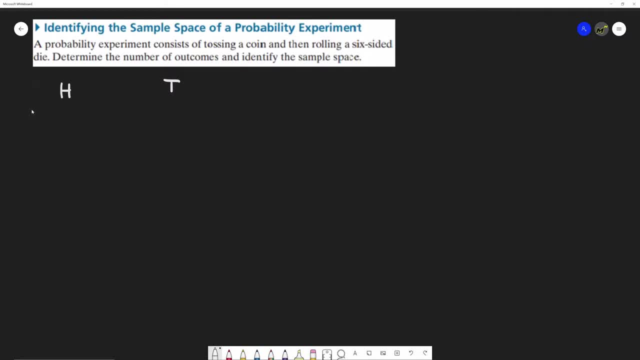 Not at the same time Your die. you can roll a one through six for a standard die. And same thing here. If you flip your coin and you give it tails, you can still have one through six on your die. Okay, So all your sample space could be 1H, 2H, 3 and a Heads 4 and a Heads 5 and a Heads. 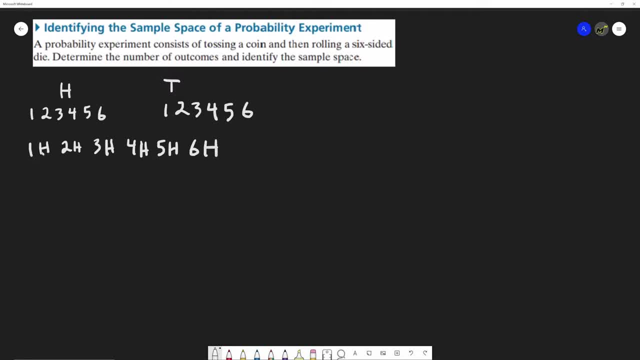 6 and a Heads. So this is saying you could roll a 1 on your die and get a Heads, flip a coin and get Heads 2 on your die and flip a coin and get Heads 3 on your die and flip a coin and get Heads. 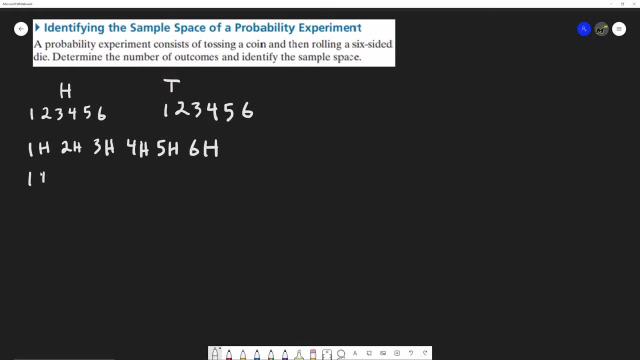 and so on. Same thing with the tails. so you could have roll a 1 and get a tails, roll a 2 and get a tails all the way. So if we list it all out, we are identifying the sample space right here. 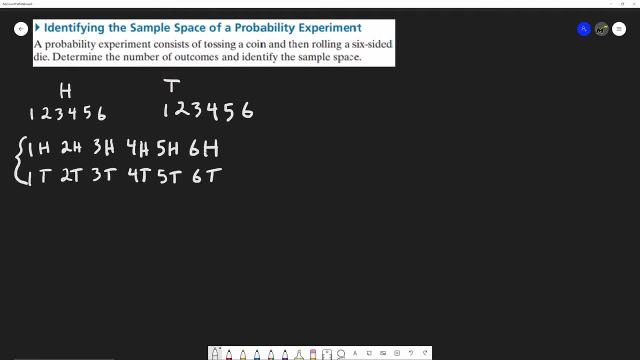 So this would be our sample space. all of this right here. 1 through 6 with your Heads, 1 through 6 with your tails. That is every possible outcome in this example. That's your sample space. Okay, Now we're going to come back to that in a moment. 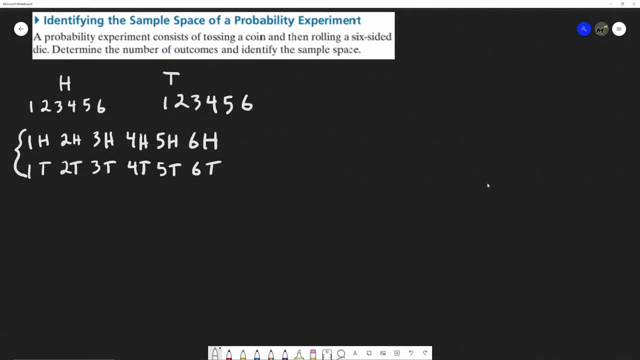 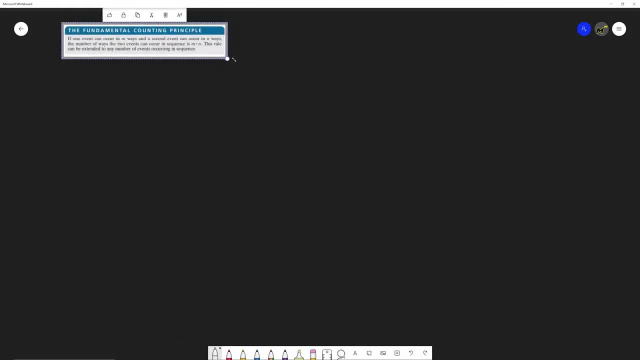 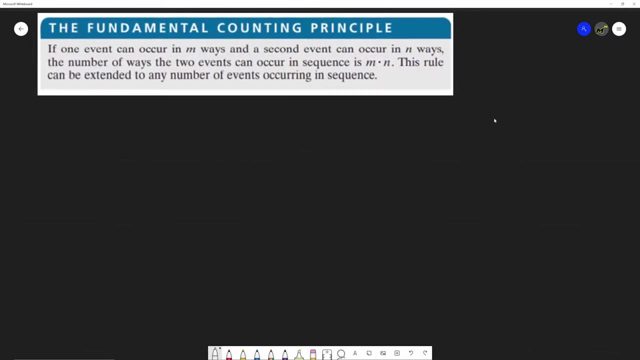 Let's go ahead and get a new term. So here we have Really important The Fundamental Counting Principle. Let's go ahead and define it. Here's our Fundamental Counting Principle, And if one event can concur in m ways, right, a number of ways, and a second event can. 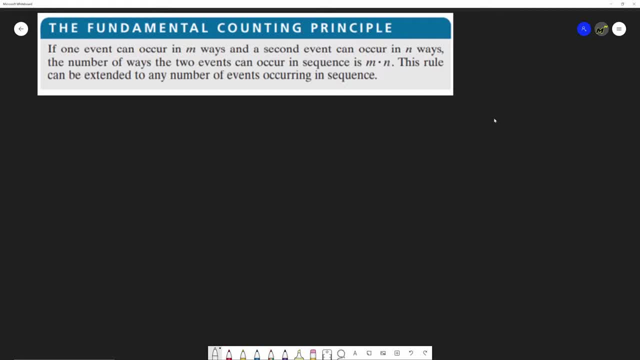 concur in a number of ways. a different number right. that means the number of ways the two events can occur in sequence is m times n. They multiply together. So that means the number of ways the two events can occur in sequence is m times n. 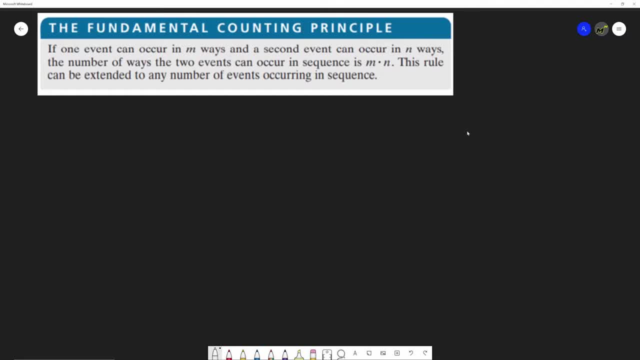 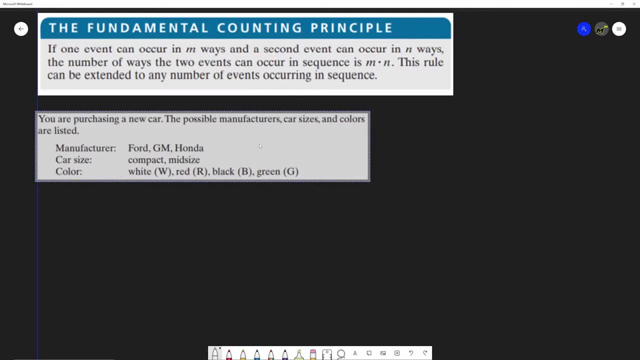 So that means more than just two, right, You could have three of them, four of them, five of them, and so on. So let's take a look at an example. So let's say you're going car shopping, You're purchasing a new car. 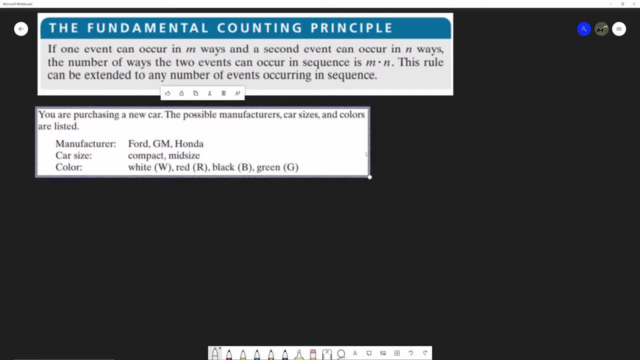 The possible manufacturer's car sizes and colors are listed. So we have a manufacturer. We're looking for three things. We narrow down our search. We're looking for a Ford, a GM or a Honda. We either want a compact or mid-sized. 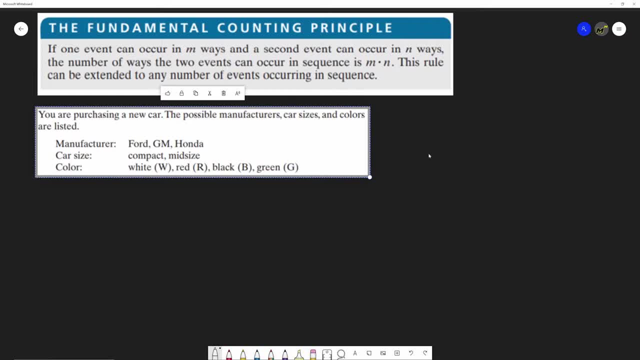 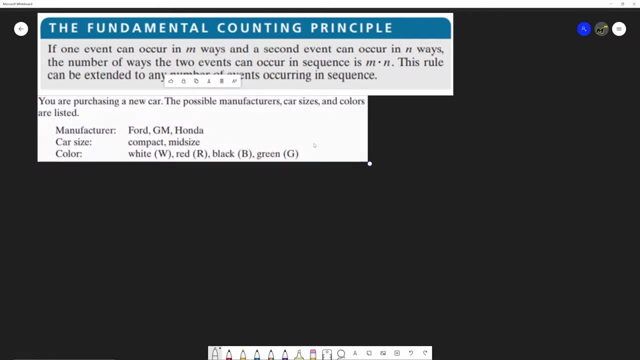 And I only want four colors: white, red, black or green. okay, If I were to map this out like draw a tree diagram, here's how this would look. So I want either a Ford, a GM or a Honda, right? 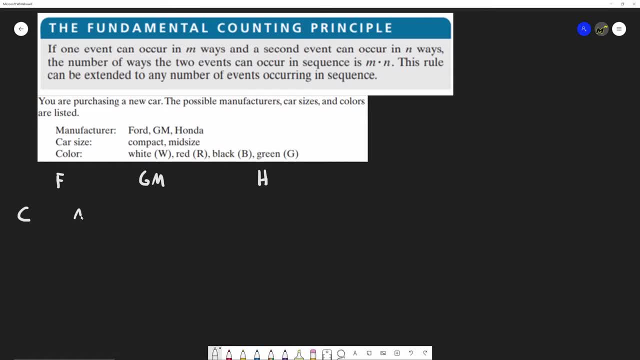 Then I either want a compact or a mid-sized. Here I want either a compact or a mid-sized, And here I either want a compact or a mid-sized, And the color I either want to have white, red, black or green. 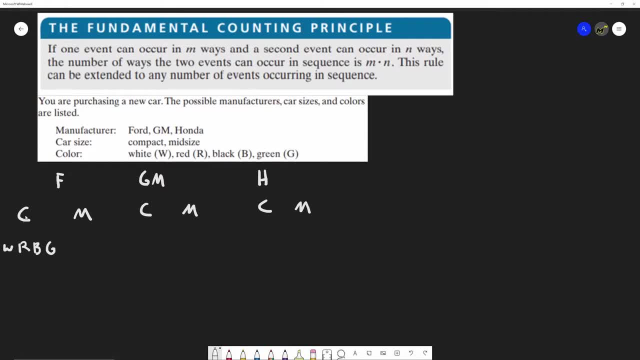 And so you see where this is going. So if I have a Ford and it's compact, I can choose between white, red, black or green. Same thing here: If I have a Ford and it's a mid-sized, I can have four colors to choose from: white, red, black or green. 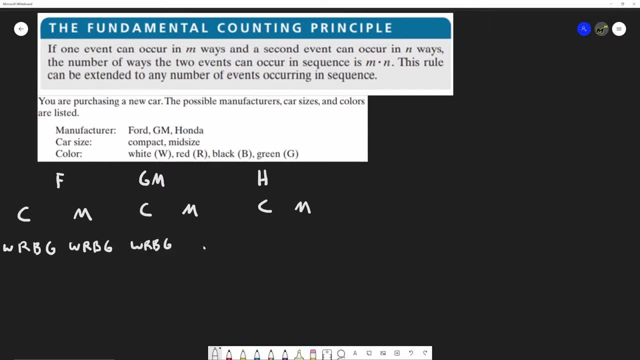 And the same thing here: white, red, black or green. white, red, black or green. And for the mid-sized here a Honda compact: white, red, black or green. And same thing for the Honda mid-sized here, four color options: white, red, black or green. 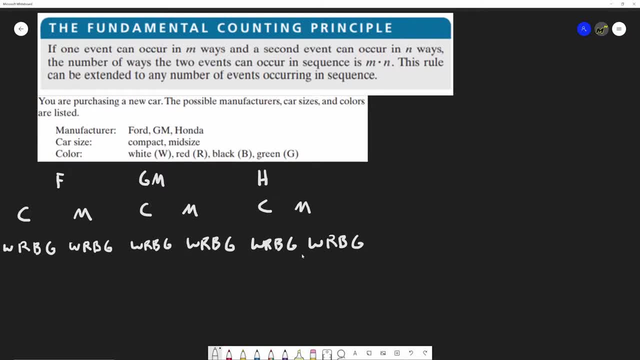 Okay, so we have four, eight, twelve, sixteen, twenty and twenty-four options. Well, drawing a tree diagram and mapping it all out like that could be time consuming. Let's go ahead and use the fundamental counting principle, which states we can multiply these different events. 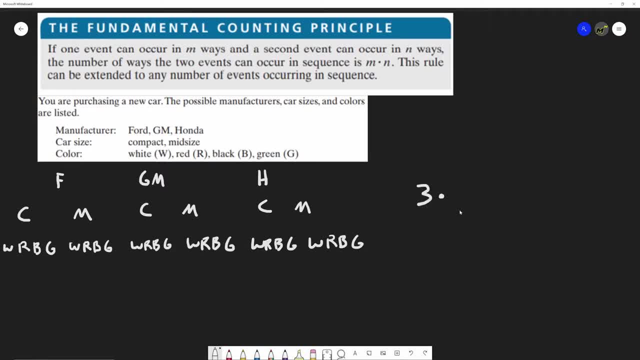 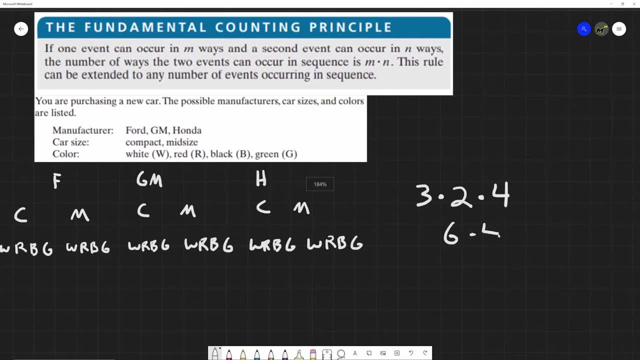 So we have three manufacturers, we have two car sizes and we have four colors. So that means three times two, we'd have six Times our fourth and we'd end up with twenty-four possible different cars, Just like we had here. we counted twenty-four options. 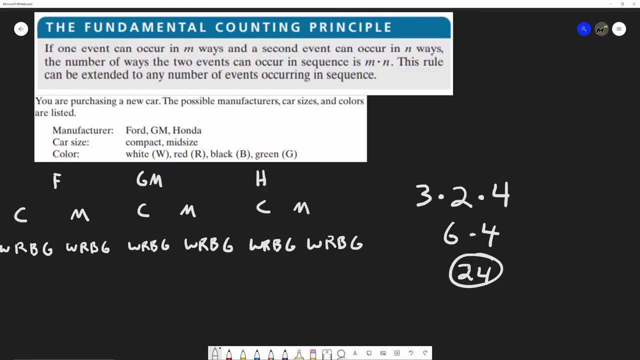 Hey, fundamental counting principle Did this in a fraction of the time to get us twenty-four outcomes. Awesome, fantastic. Let's go ahead and use that. It's much more efficient. Okay, So this is where you could go back, and so we identified our sample space. if you wanted to map them all, 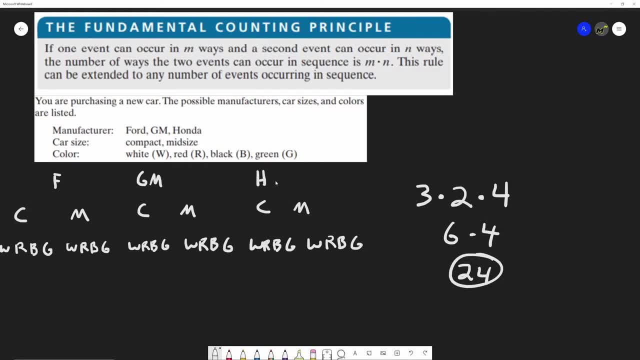 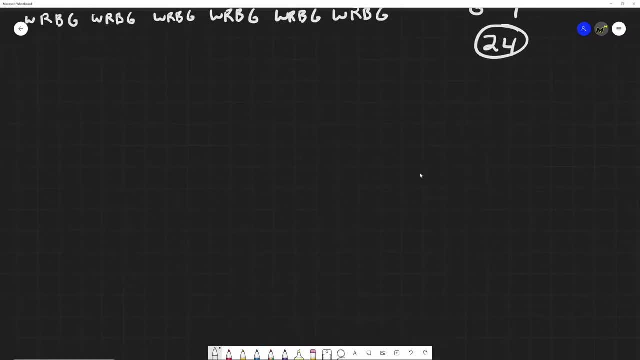 That's our sample space, right there, Every possible outcome on a tree diagram. I didn't draw the arrows. That would be that Fundamental counting principle. That's that Last time. Okay, Let's use more of the fundamental counting principle. 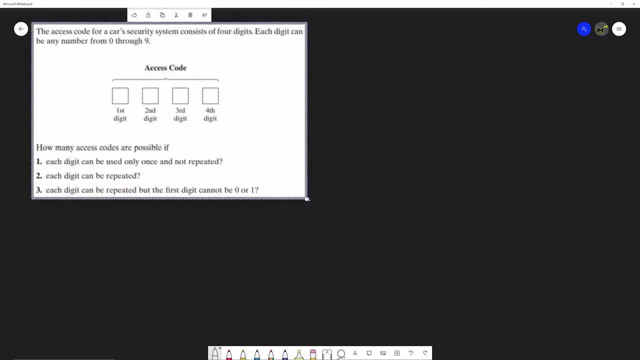 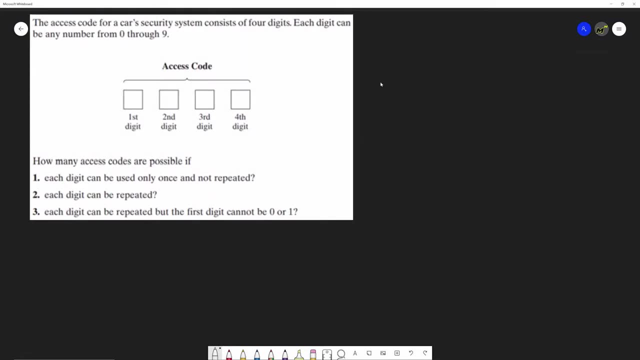 Next example: The access code for a car security system consists of four digits. Each digit can be any number from zero through nine. Okay, So we have four digits, zero through nine. How many access codes are possible if number one? each digit can be used only once and not repeated. 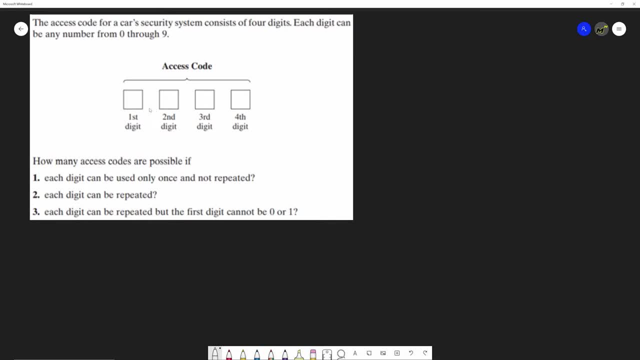 Okay. So let's think about this: We have four boxes here In zero through nine. well, let's see Zero: one, two, three, four, five, six, seven, eight and nine. Okay, So we actually have ten numbers, right. 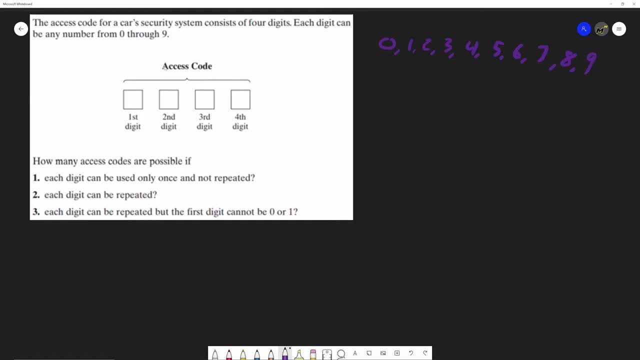 We have ten options. Zero counts Once a number is used. it's no longer an option Right now. we have ten numbers available to us for our first digit, so I can put in ten there, Right Number one, first digit. I can have ten options. 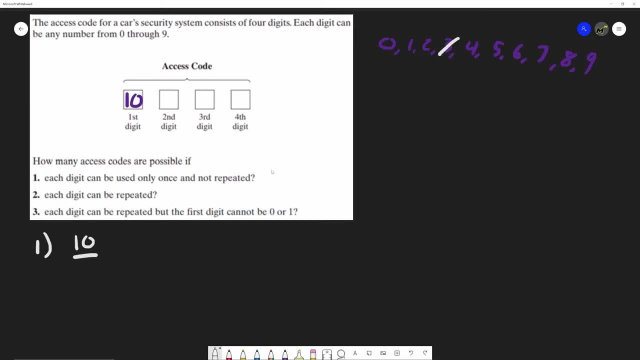 Let's say the first digit is a three. Well, how many digits do I have available now for the next one? Because they can only be used once and not repeated. so that means that I'm going to I'd have 9 for the next one, so the next digit I'd have 9. and then, if I say 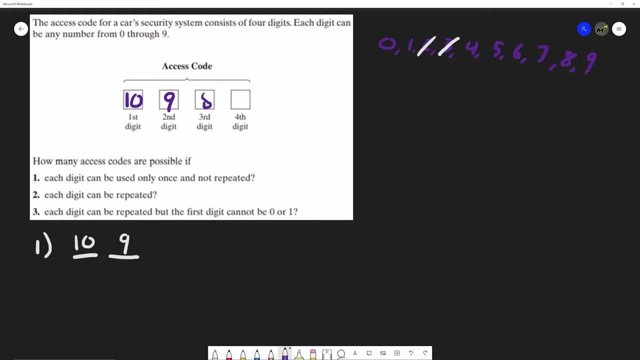 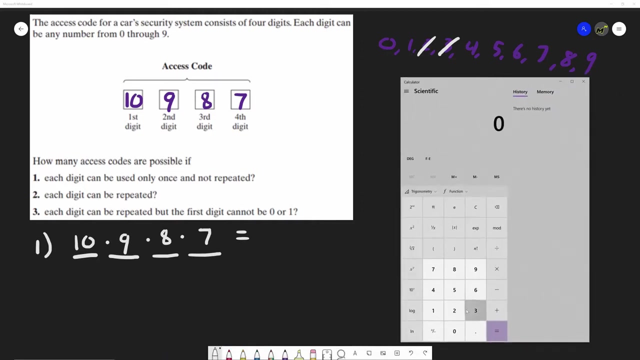 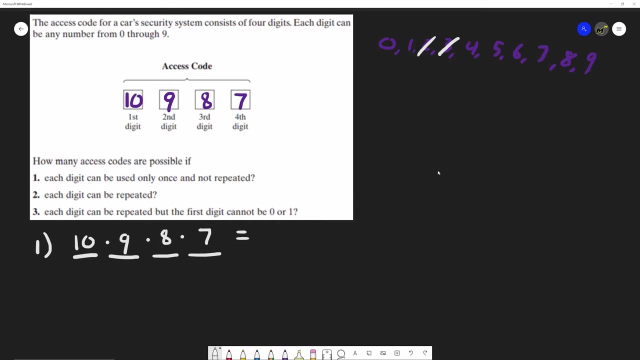 that's a 2. well, now I have 8 numbers available, and then I have 7, and we're using the fundamental counting principle. so you're actually going to multiply 10 times 9 times 8 times 7, and that would give you so 10 times 9 times 8 times 7, so 5,040 ways this code could be created. 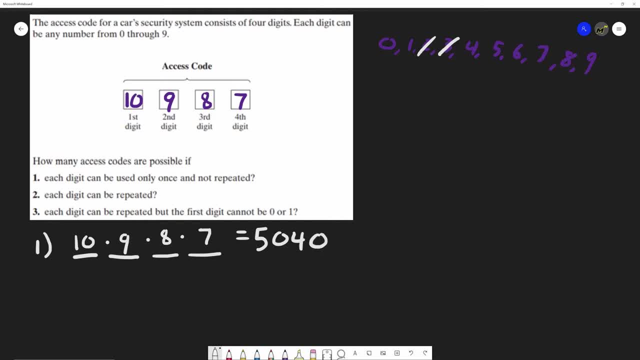 so with these parameters, you have 5,040 different codes that you could create. well, let's look at the second one. so each digit can be repeated. okay, so that means we're not constrained. so if you pick a 3 here, it's no longer going to be crossed out. 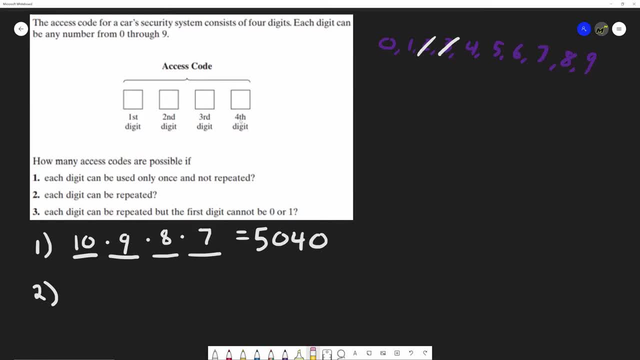 you can use a 3 in the second digit and the third digit and the fourth digit if you wished. so that means we'd have 10 numbers available to us in the first one, we'd have 10 numbers available to us in the second one, 10 numbers available in the third one and 10 numbers available in the fourth one. 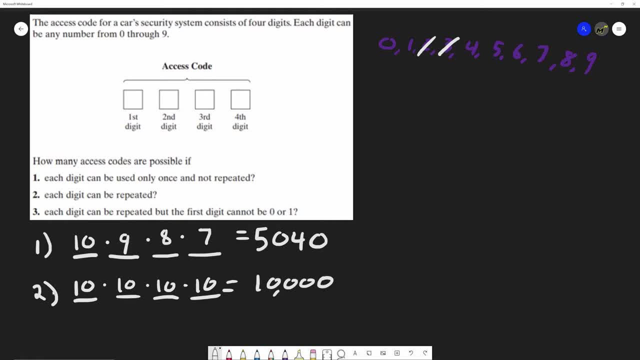 that'd be 10,000 possible options for your code. so if you think about an iPhone, right, yeah, they used to. I think they use six digits. now a lot of people use six digits, but early iPhones it was time to have a four digit code. this was how many choices you had. you had 10,000 possible codes and then their 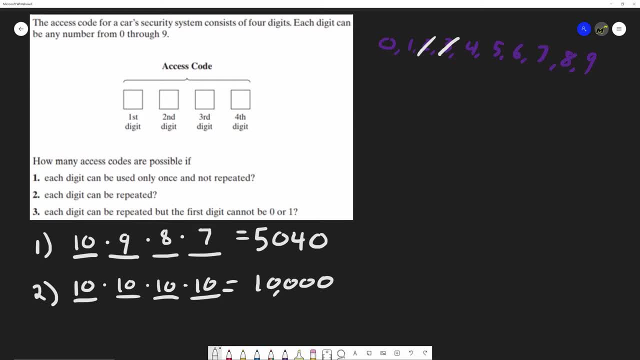 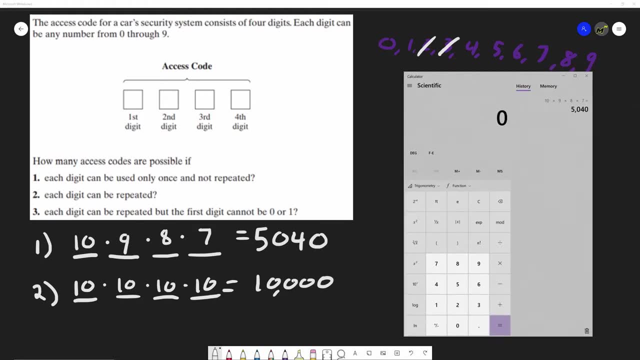 security measure was you could only try it 10 times before it erased all your memory. so here let's do that real quick. so if you were on an iPhone back in the day before, you had six digits, we had 10 tries out of 10,000. if someone's just 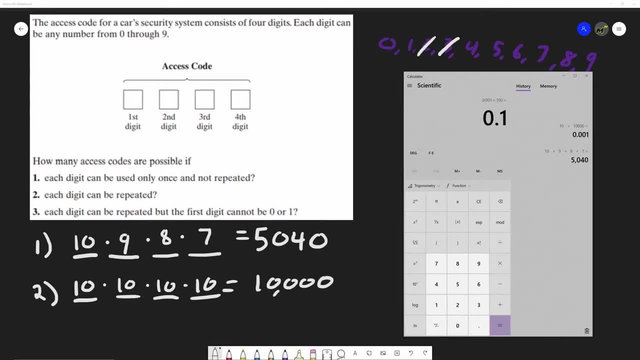 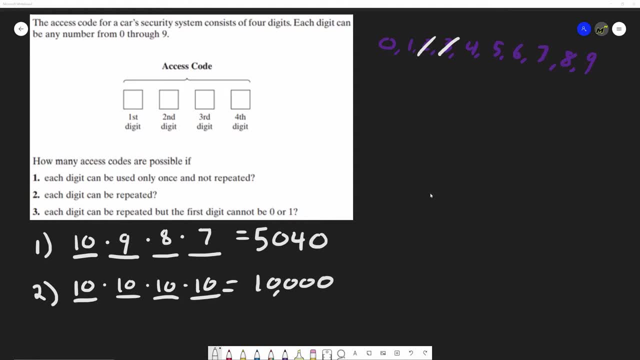 blindly guessing, they'd have a point one percent chance of getting it right. if they're just blindly guessing, all right. move on to this number three. each digit can be repeated, but the first digit cannot be zero or one, so they're putting some constraints on us here. 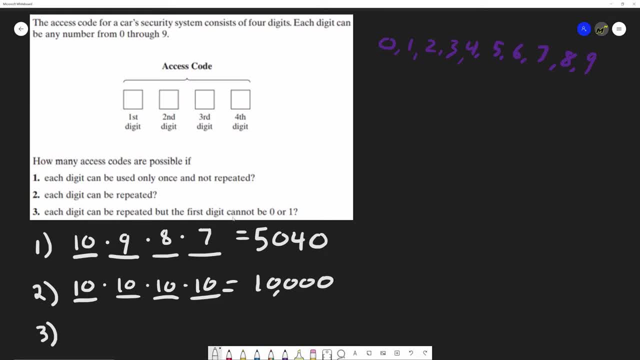 this time they're saying: hey, you can't use a zero or one in the very first digit. that means first digit. we only have eight numbers available to us. so there you go, eight. and then we have a no constraints for the rest of them. so that'd be ten. the third digit we have: ten. 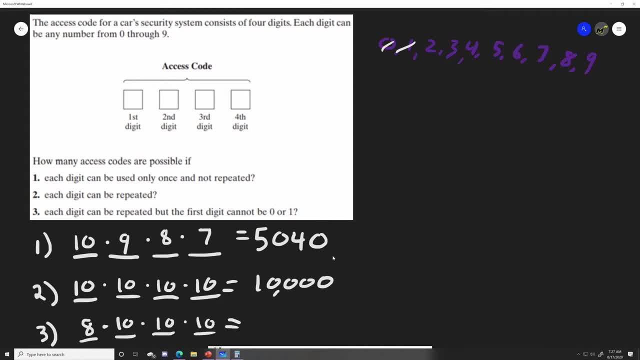 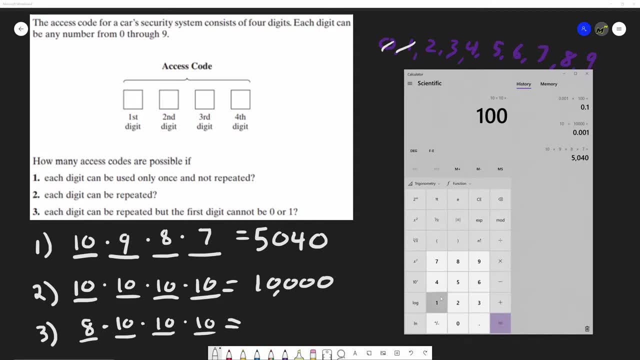 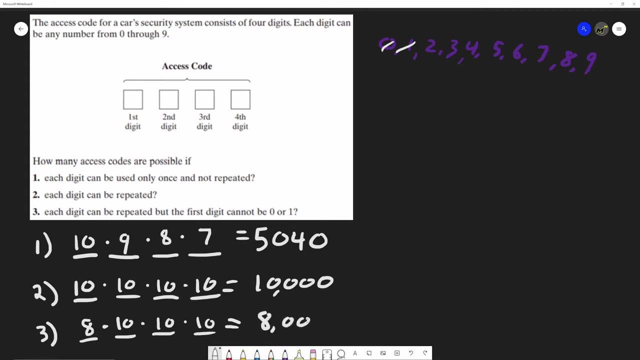 options and the fourth digit. we have ten numbers available to us. let's see so: eight times ten times so, thousand times eight, eight thousand, right times eight. yeah, eight thousand. I've done for you. anyway, here you go so, this concept that we're using the fundamental counting principle. the setup is a. 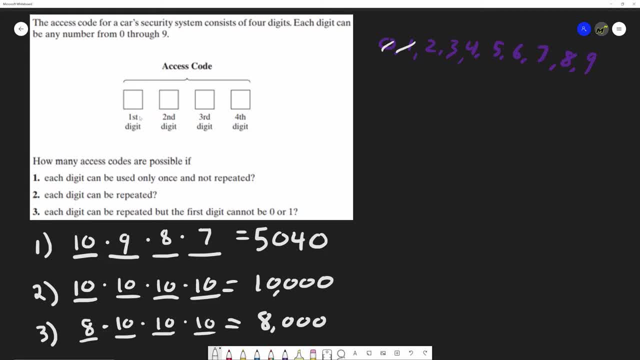 little different, because we're talking about a code and you have to really think about: hey, how many digits, how many options do I have here? what's my sample space? let's take it a little of both worlds that we started with. you have to figure out your sample space. how many numbers do you have available to you? how? 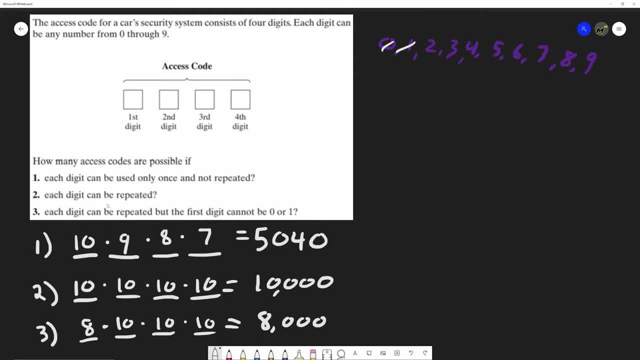 many numbers do you have available to you in each digit? can you repeat it? can you not repeat it? so the parameters really matter and of the context in which you're looking at really matter, because that multiplying isn't too difficult. however, you got to make sure you're thinking of these parameters and 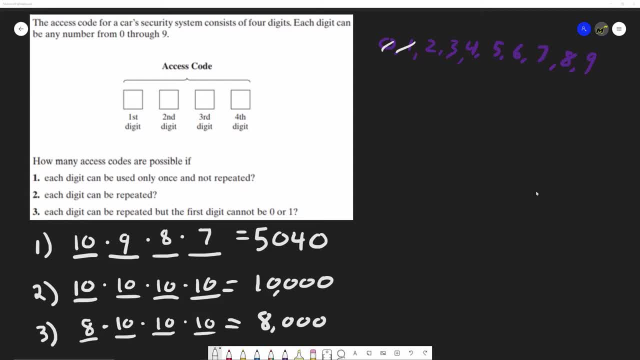 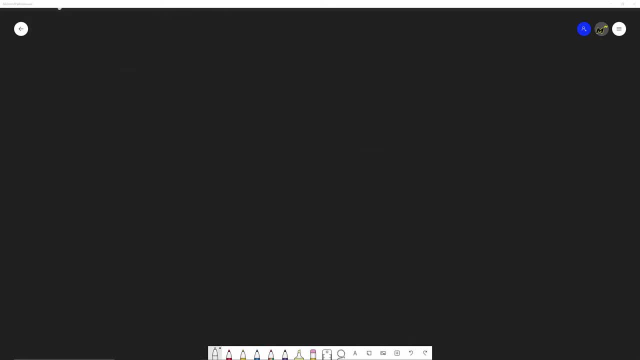 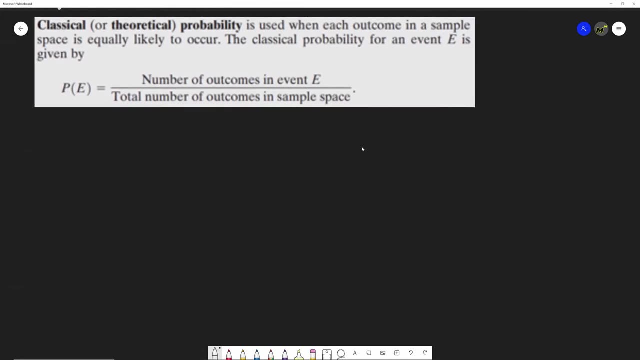 you're getting those correct. all right, let's move on to the next item. so here's something we have, classical probability, and so it's basically I use. when each outcome in a sample space is equally likely to occur, a classical probability for an event E is given by this formula, so we have number of events. 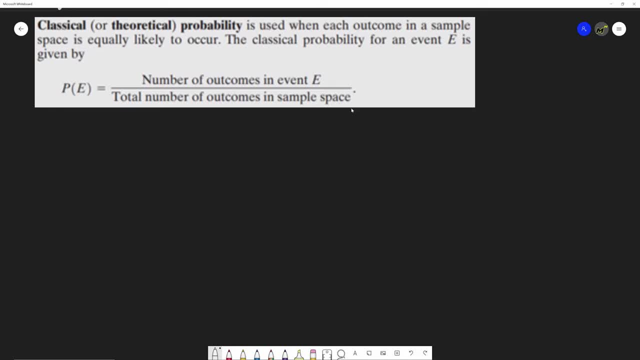 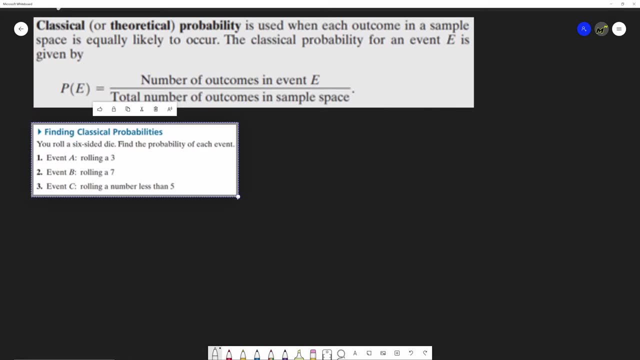 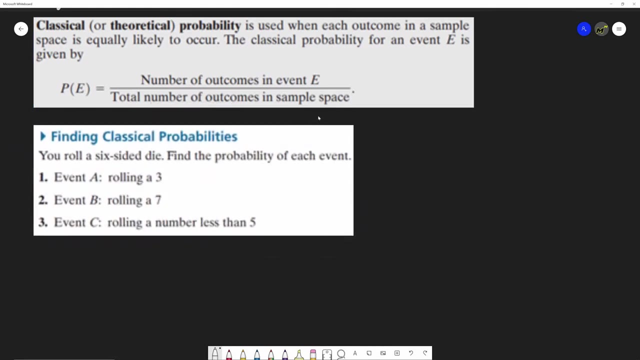 on top, divided by the total number of outcomes in the sample space. so best way to do this, let's just do a couple examples. let's say you've rolled a six-sided die. find the probability of each event okay. well, number one here, rolling a three you have. there's only one side of a six-sided die. 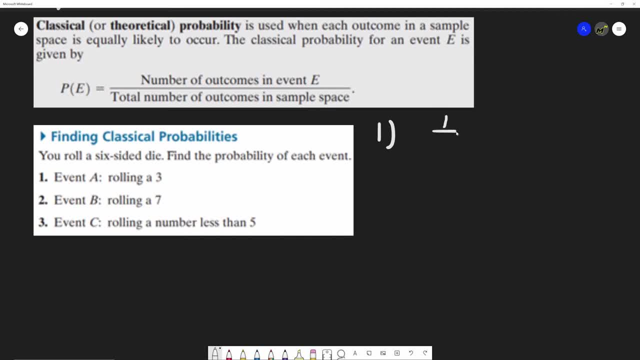 that's a number three if we're talking about a standard one. so we have one out of six possibilities. that's it one out of six. you can change that two percent if you'd like, but we'll keep it as one out of six. let's see. 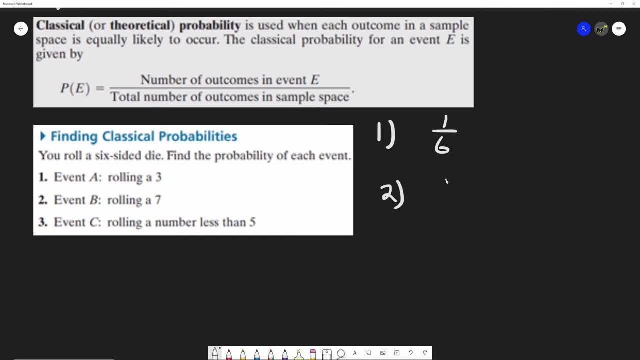 rolling a seven. well, on the six-sided die there is no number seven, so that'd be zero out of seven. there's no possible way to get a seven, unless of course you had a second die. then that's a different, a different problem entirely. and event C rolling a number less than five. oh so here we. 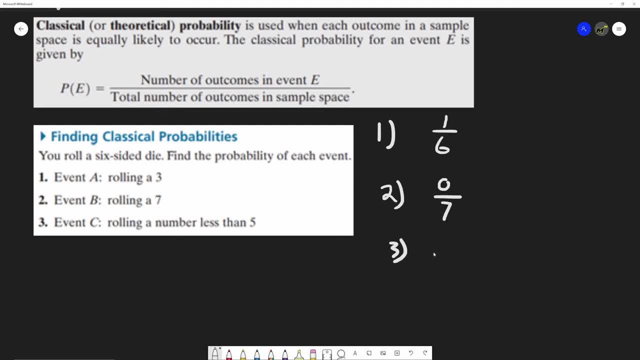 have more than one outcome. we have a subset of outcomes. it's not entire, give all the outcomes, but rolling less than five. so let's see: a one is less than five, so is a two, so is a three, so is a four and a five is not going. 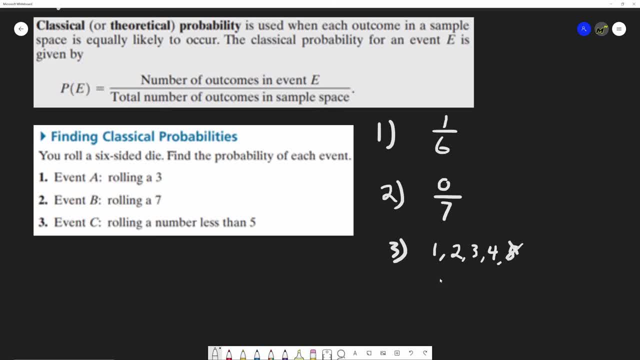 to count, because they say less than five, which means we're not going to include it. so we have four out of six possibilities. you can simplify it and say it's two-thirds and then, if it's a percent, yeah, you could say it's sixty six point six, seven percent. we'll leave it here as a fraction, all right. next,